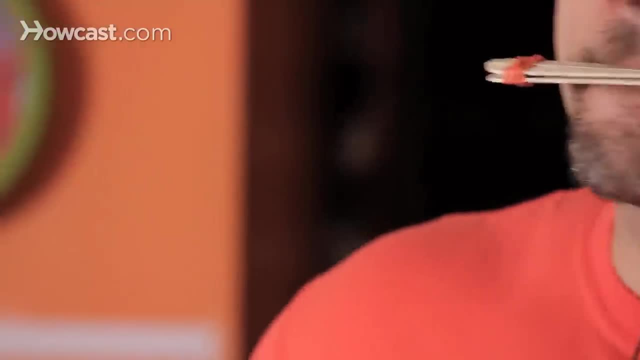 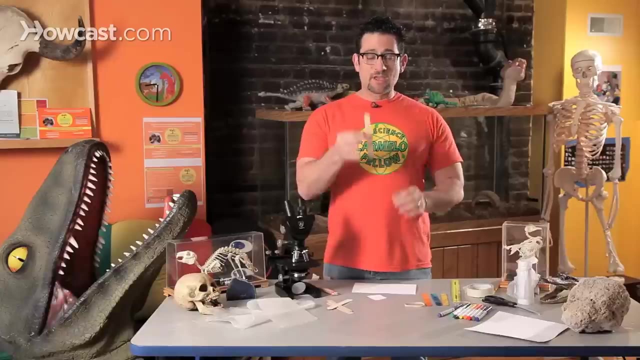 And I'm going to make an amazing instrument using nothing but tongue depressors and rubber bands. Sound like a rapper, rapper, Carmelo. Now step one is you take a rubber band. okay, I think a thicker rubber band works great for this experiment. 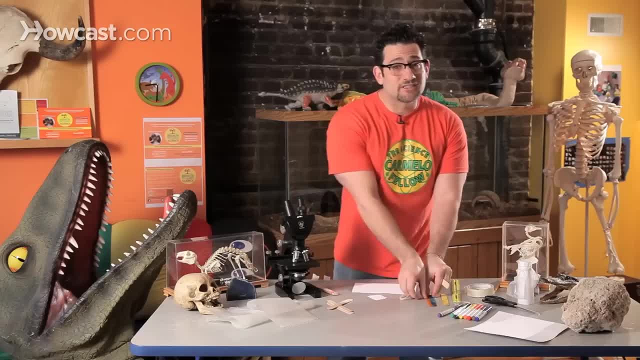 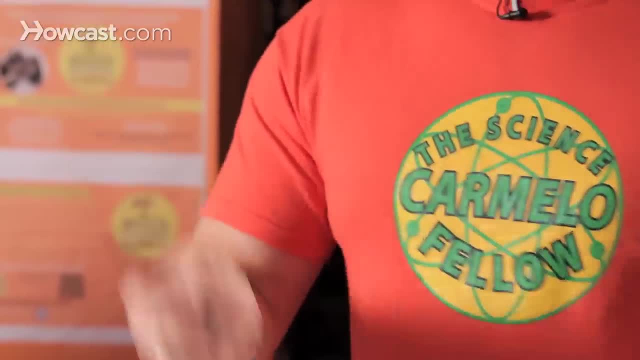 And I take this tongue depressor and if you wanted to, actually you can color your tongue depressors so that your harmonicas look amazing. okay, I'm just going to make mine non-colored, but if you wanted to use markers, you could make. 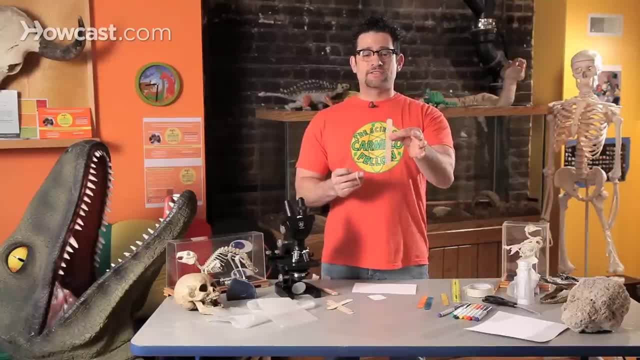 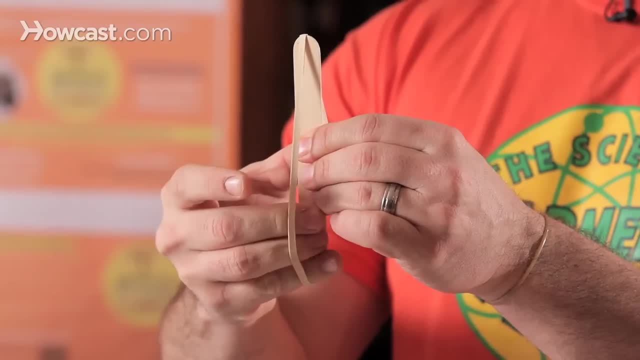 them colored, You could make them look fun, because actually, look you store-bought these. Step one is: take your tongue depressor large rubber band for this step and you can take it very easily. just wrap it around your tongue depressor, just like that. 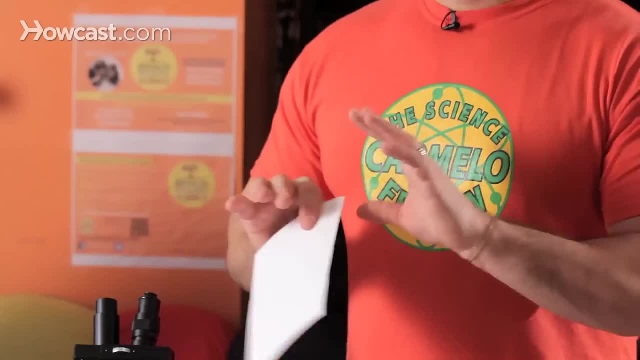 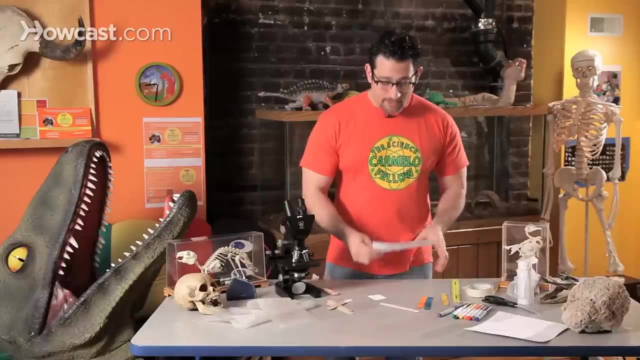 Easy step. Step two: again card stock. I don't like typing paper, I don't like computer paper, I like using card stock. It's a little thicker and it makes the experiment work that much better. And I'm going to cut out a piece, two inches, two inches by two inches. 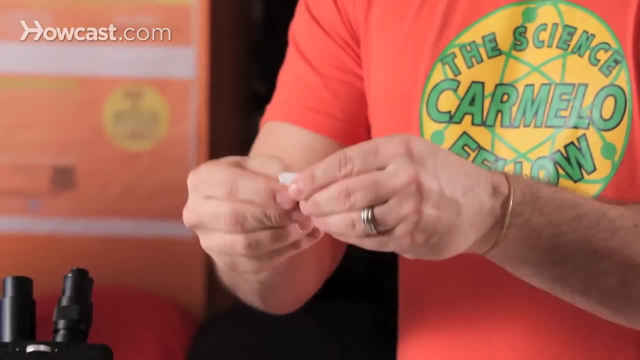 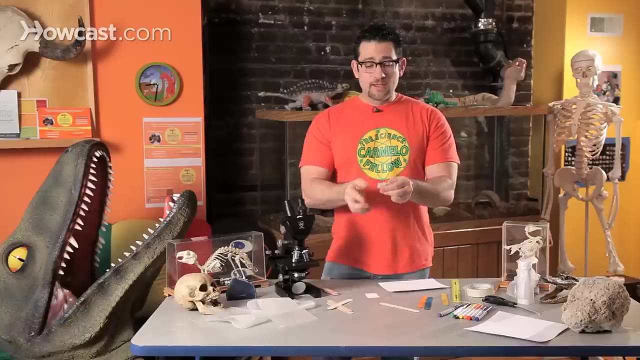 So there's your math measurement, okay, And I take it and I'm just going to fold it, fold it and fold it. So I'm going to take the square and I'm going to fold the square three times. I'm going to take a piece of tape that I'm just going to roll around so that the tape 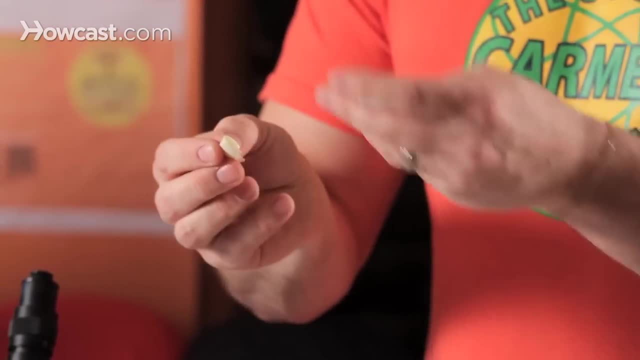 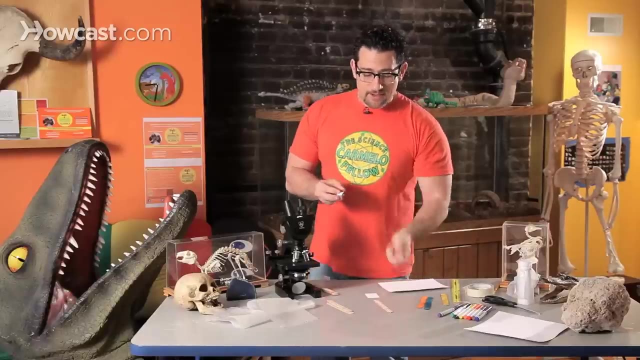 is sticky on all of its sides. okay, Take the piece that I cut out, put it on the tape. I'm going to take my second tongue depressor, not the one with the rubber band, and I'm just going to tape it, not at the end. 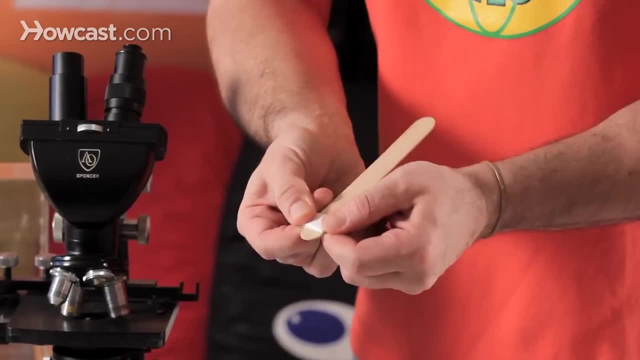 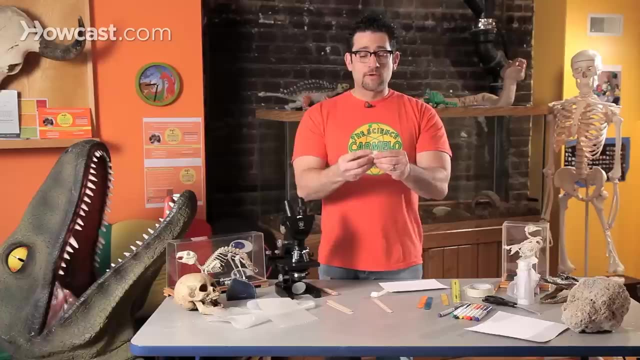 I'm going to leave a little bit of space just like that. And now I'm going to do the same thing twice. I'm going to take another two inch square, remember, two inches by two inches by two inches. I'm going to fold it, fold it twice, fold it three times. 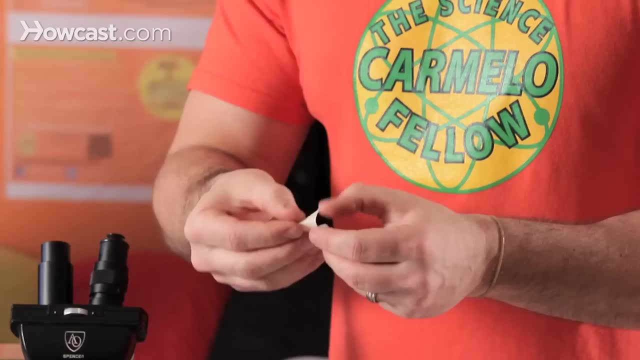 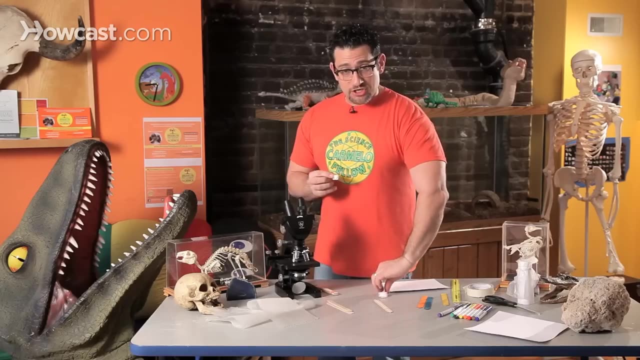 It's exactly the same step. Take another piece of tape, roll it so that it's sticky on all of its sides, and you're going to make this exact. it's going to be symmetrical, It's going to look exactly the same. you're just going to do it on the other end. 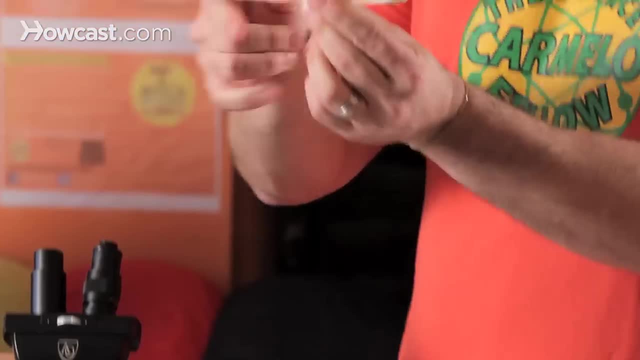 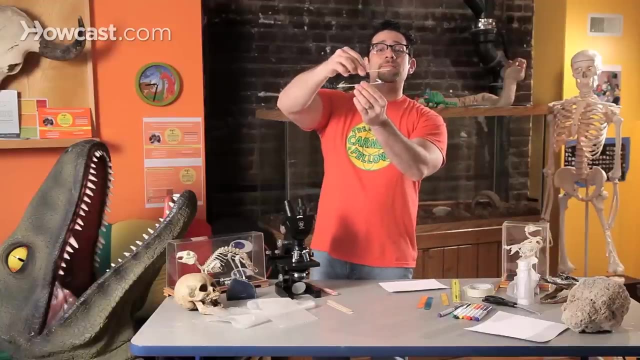 Again a little bit of space, and now I have that Kind of looks like you're going snowboarding, right, But we're not. Now I'm going to take what I did: step one, Okay, step two, and I'm going to make a stick sandwich here and I'm going to push it together.